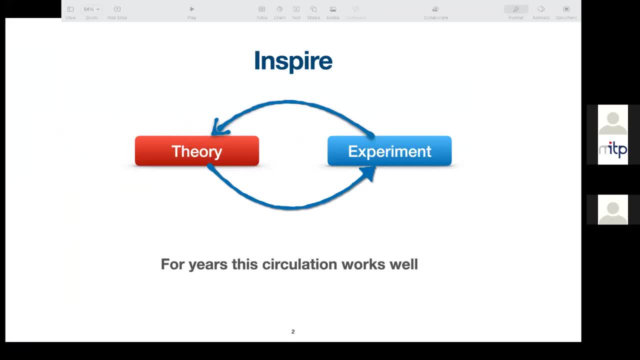 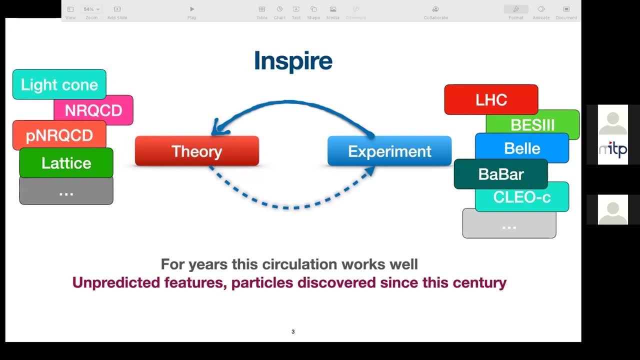 The theory and the experiments inspire each other and for years this circulation works well. However, since this century, the A lot of unpredicted phasers or particles are discovered by RCB, Bell, Barbar, Bessie and Cleo, and a lot of those, a lot of those particles and phasers could not be described 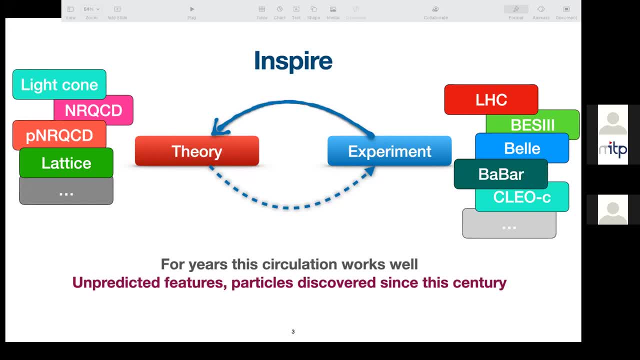 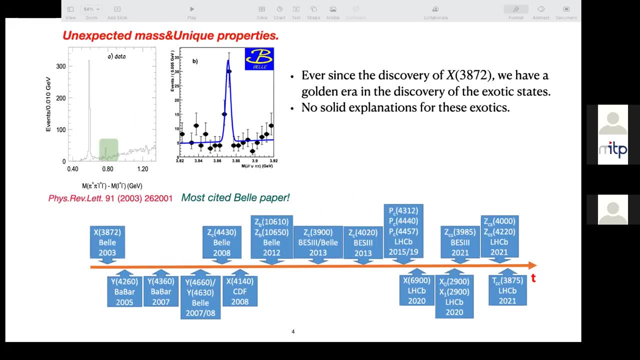 well with conventional theory pictures. All these stories Start from the discovery of X-372, which is the first observed, Which was first observed in the environment mass of a Pi Pi JSI. The unexpected mass and the unique properties quickly grabbed everyone's eyes. since the 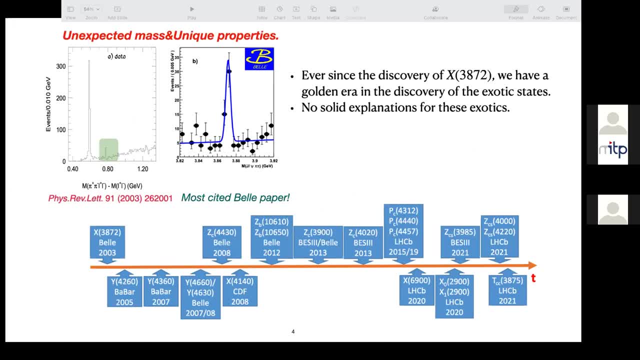 Once the We, Once X-372 is discovered. Ever since then, there are the Y, Not only X particles, the Y particles, they Even the pentaquark or the double-chamber, double-chamber biome states are observed. 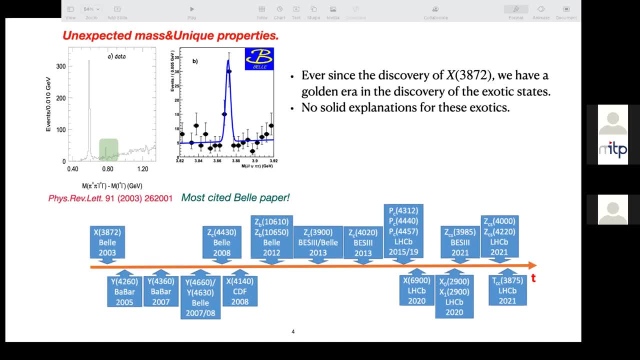 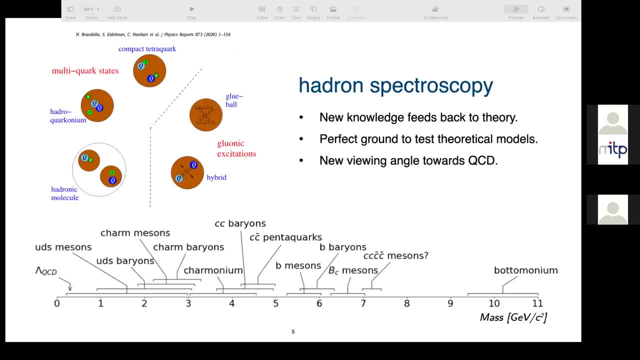 Until now, this observation of X-372 has been the most cited Bell paper, So So. So So, To explain those states that we observed, there are a lot of Models to. There are lots of models, for example, the compact tentacle quarks, the hydrogen quercunium. 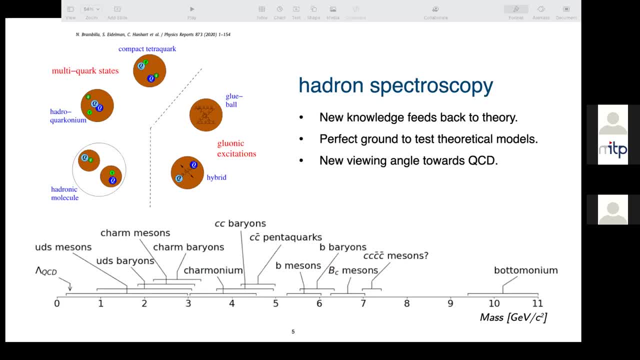 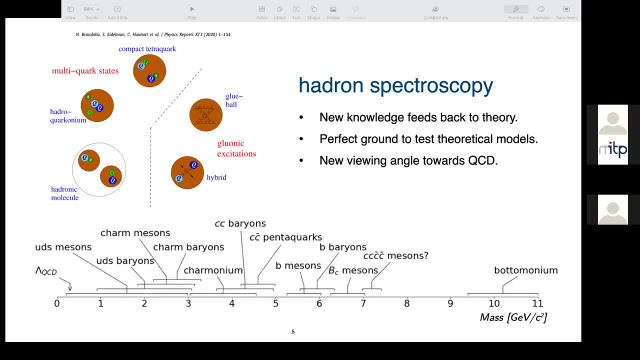 Hydron, Hydron, Hydron Hydron back to the theory, and it's also a perfect ground to test the theoretical models. The hydron stratoscopy also provides a new viewing angle towards the QCD theory. 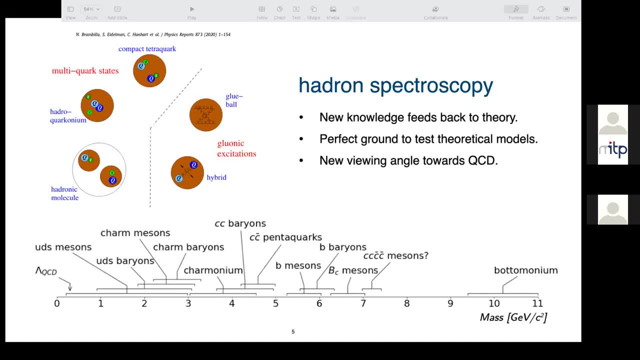 In this picture you can see that we showed the mass scale of the stratoscopy for the hydrons. For the lower mass we could study the biomes and the energy goals. The ones we have are chamronium and bortimonium. 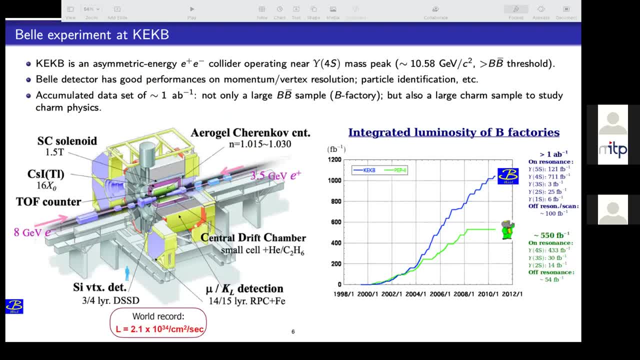 Firstly, let's have a quick review of the Bayer experiment. The KKB is an asymmetry E-plus, E-minus collider operating near the open-source mass peak. The world record of the luminosity is 2.1 times 10 to 34.. 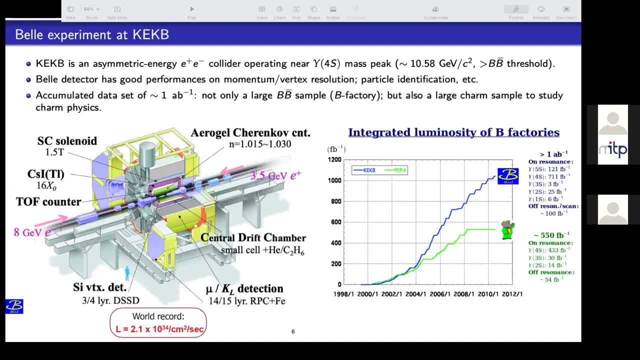 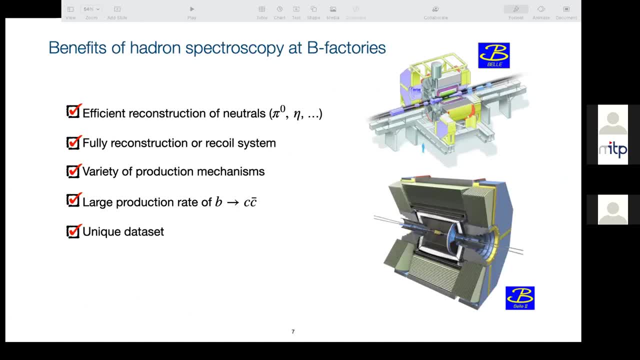 The total integrated luminosity is almost 1 eV. The benefits of the hydron stratoscopy at the Bayer factory is that the Bayer factory has efficient reconstruction of the neutrals and we can also have a fully reconstruction of the system. There are varieties of production mechanisms to produce the different hydrons. 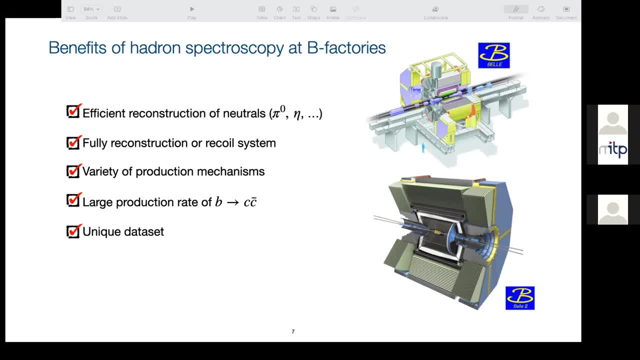 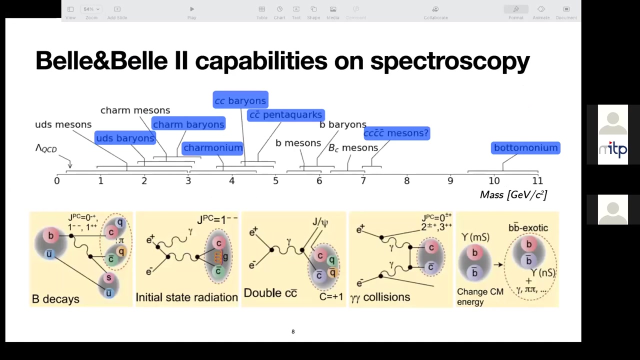 the large production rate of B2CC-bar also provides a solid ground zone. The unique dataset on the Bayer PyGory Food and Research Laboratory also provides a solid ground zone for cutting of deaths. a unique view to study the hydron spectroscopy and the QCD series. 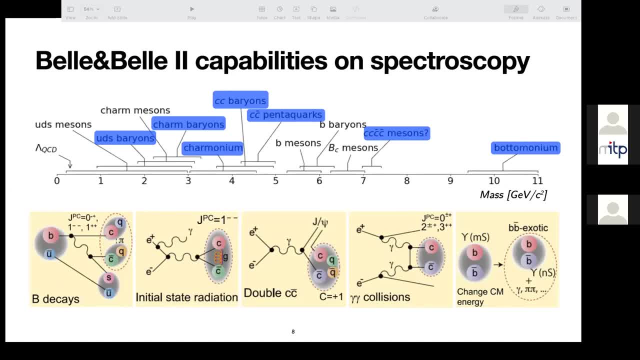 Here is the Beo and Beo2 capabilities. on the spectroscopy, The low energy particles, we can work on the UDS bionth, the charm bionth. Then, as the energy goes down, we can have a charmronium or the Cc bionth, Cc-brite pentaquarks or the double charmronium. 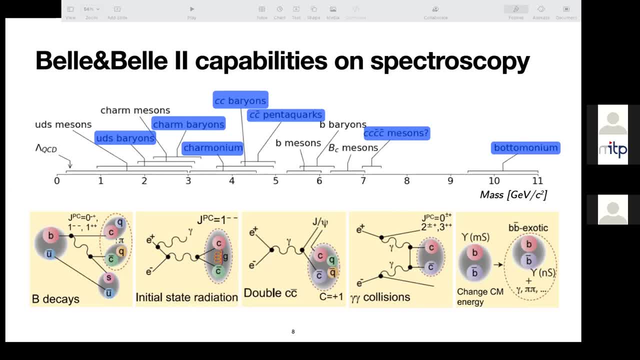 particles or the botmonium particles. We have five different production mechanisms for the quarkonium states, including BDKs: initial state radiation, double charmronium production, two photon process and the PROMPT automonium production in the E plus, E minus annihilation. 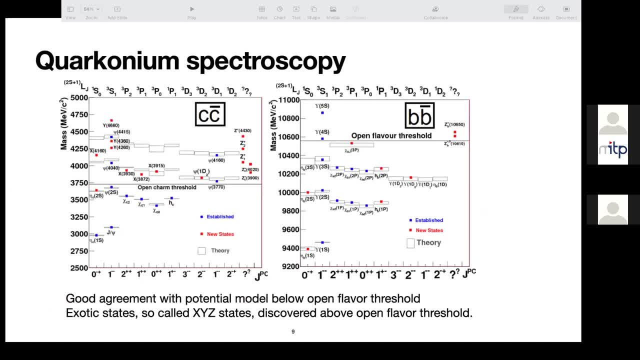 This is the quarkonium spectroscopy that we have. We have a good agreement with the potential model below the open flame, But for the particles above the open flame threshold, the exotic state, which is also called XYZ state, they do not agree with the position model or, even worse, some of those are not even. 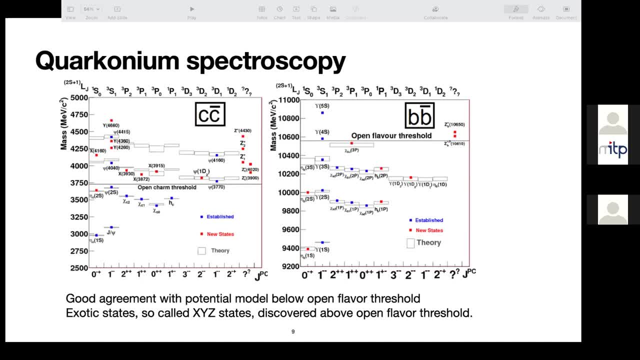 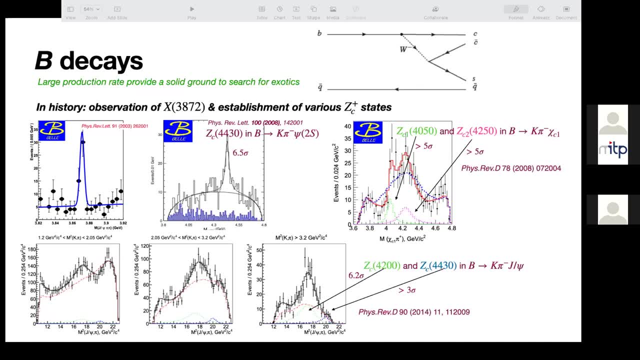 predicted, Then let's focus on some results that we have already achieved. Firstly, the BDKs. The large protection rate provides a solid ground to search for the exotic states In the history. the observation of X-372 is, of course, a great success, and we do not. 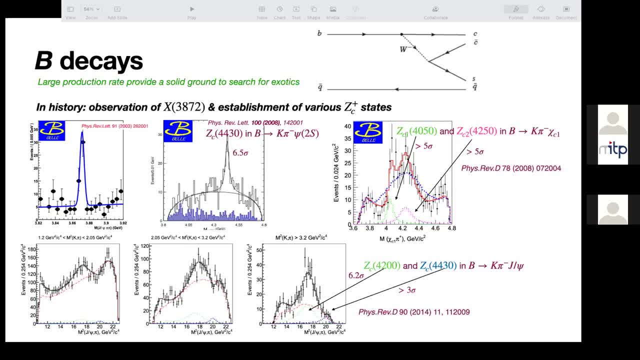 need toInteligently add data as want to track a particular or even softer defective state, such as zc4430.. The ZC4050, ZC4250 were also observed in B2-keypad KC. The significance are all greater than five and amplitude analysis. 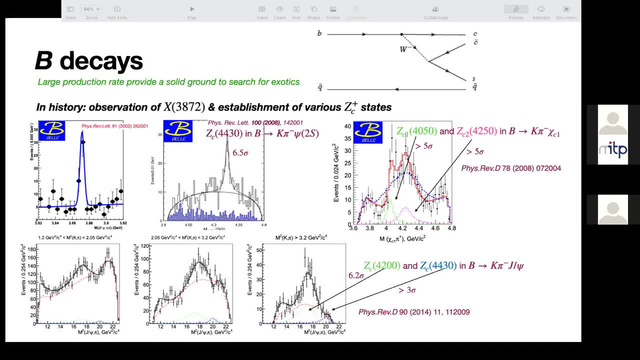 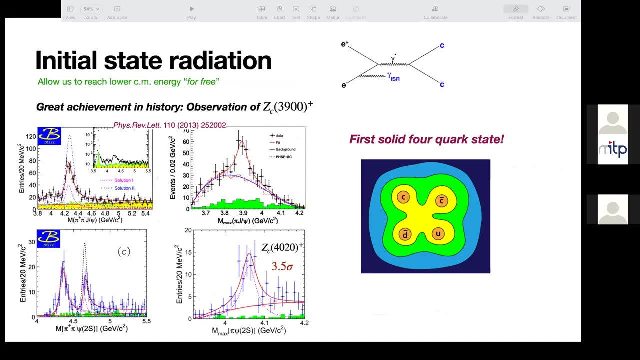 is performed to the B2-keypad JSI, and the signal of ZC4200 and ZC4430 are also found For the initial state radiation. this process allows us to reach lower center of mass energy for free. We also achieved a great success in the history. 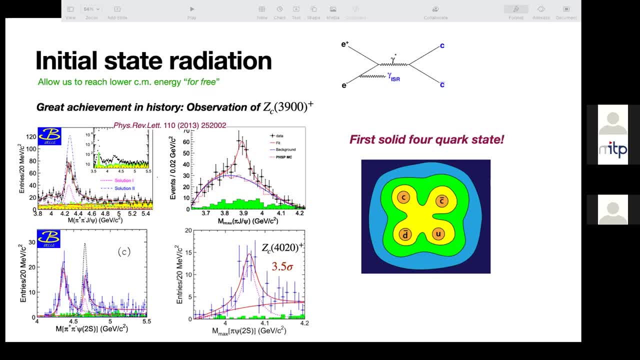 which is the observation of ZC3900.. This is the first solid for quark state that we have observed. This is the first thing. in the e plus, e minus goes to pi pi JSI and on the one pion with JSI in random mass. 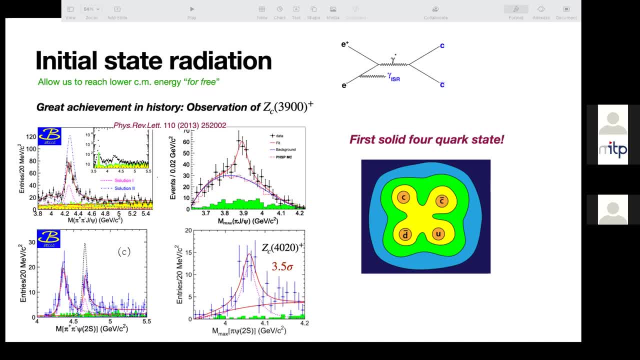 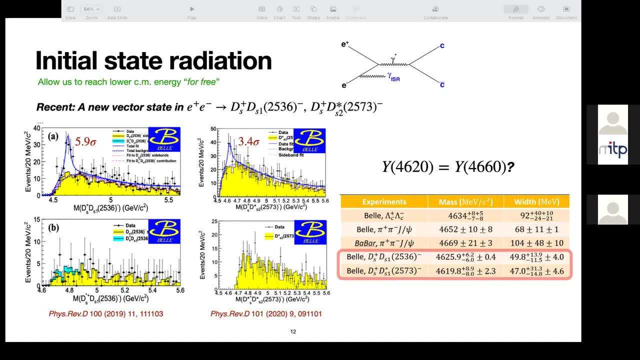 And I have evidence of this. ZC4020 was also found on pi psi 2s in random mass. Recently a new vector state in the e plus e minus goes to ds ds1, ds ds2 star is observed. So on the random mass of ds ds1, you can see a clear 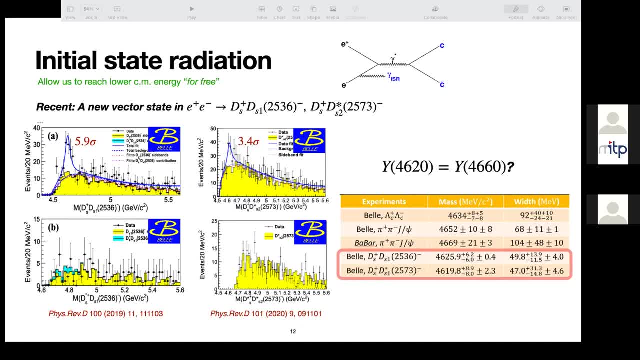 signal with a significance of 5.9 sigma is found And on the environment of d sub s, ds2 star, 3.4 sigma evidence is found. The mass of this new vector state is measured around 4620 MeV. It's quite. it's quite close to the so-called y 4650.. 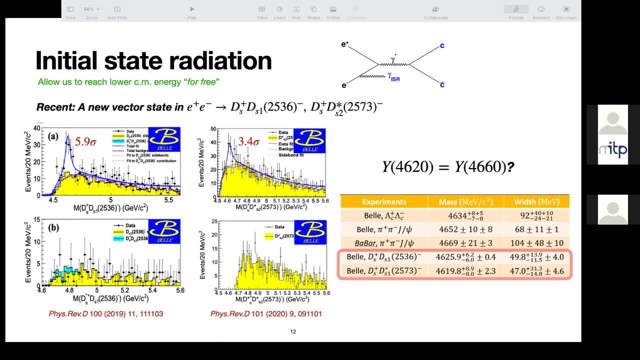 But you, if you look at the error of this, if you look at this, the error of this state, it's quite far from the. it's like three sigma far from the so-called y 4660.. We still need a lot of the studies. 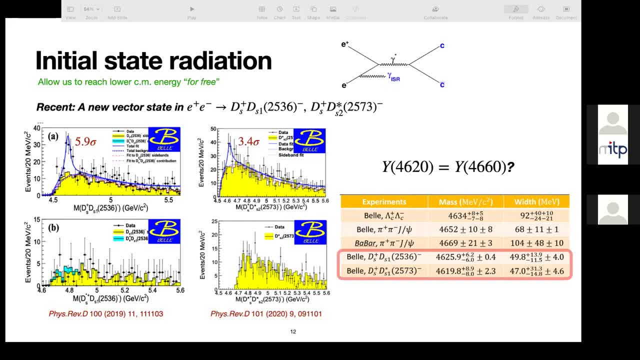 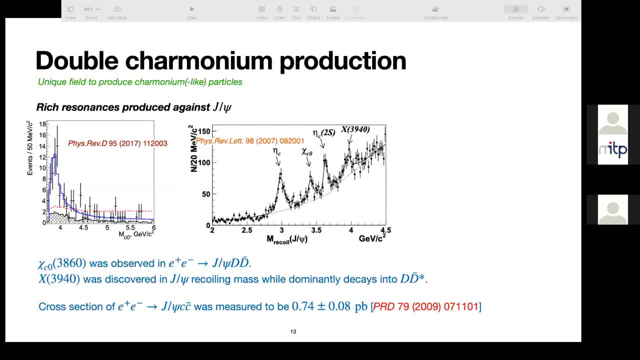 That is to separate is whether this is some state or not. The double Chamonix production is the unique field to produce the Chamonix or Chamonix like Chamonix, like particles. KC03860 was observed in the e plus, e minus goes to d bar. 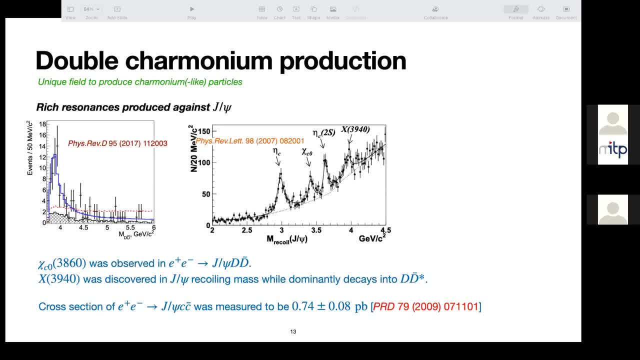 And the X3940 was observed in the. So I said you call your math with which is dominantly decayed to dd star. According to this study, the cross section of the double Chamonix production with, with the contain, the JSI is measured to be 0.774 inverse. 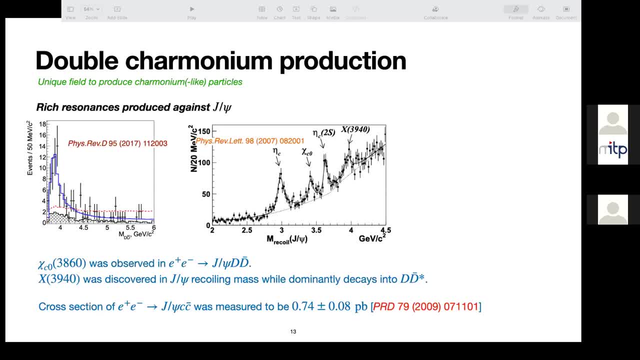 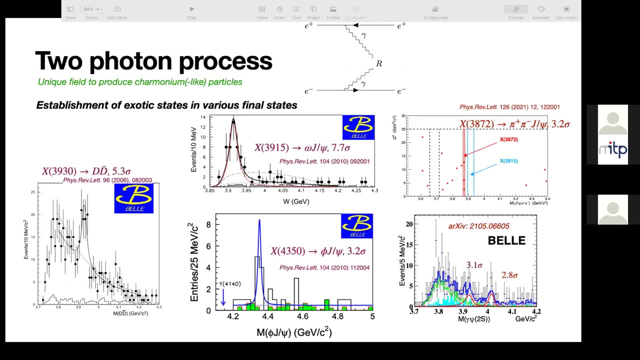 p bar, which means we there will be a rich. richness will be produced against JSI If we have more data collected. on bill two, The two photon process also provide a unique field to produce the Chamonix, or Chamonix like particles. 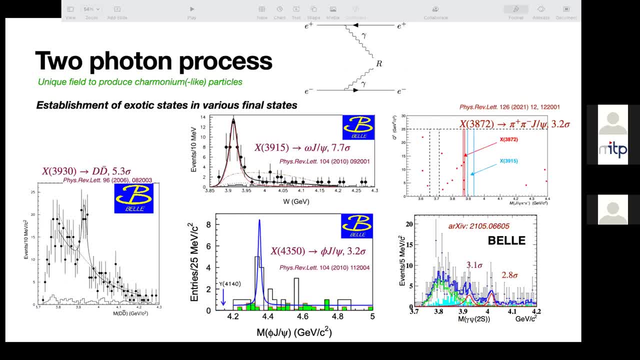 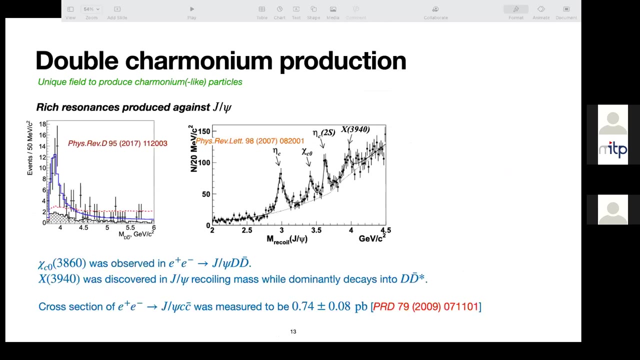 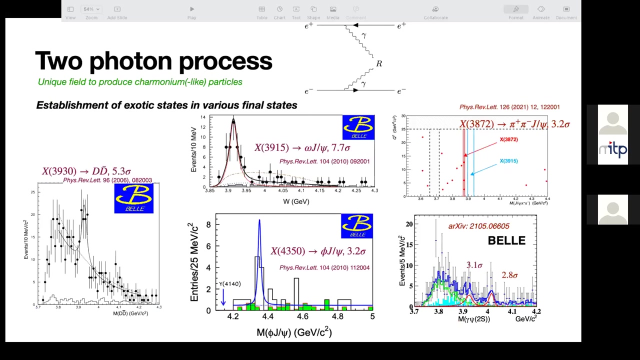 In this process, the a lot of exotic states are established in various final states. Firstly, is the X3930 to dd bar. You could, you could compare with. you can compare this particle with the previous X3860 and 3940. You can see that they are. this is, this is not the math of this. X3930 is not consistent with the 3860.. 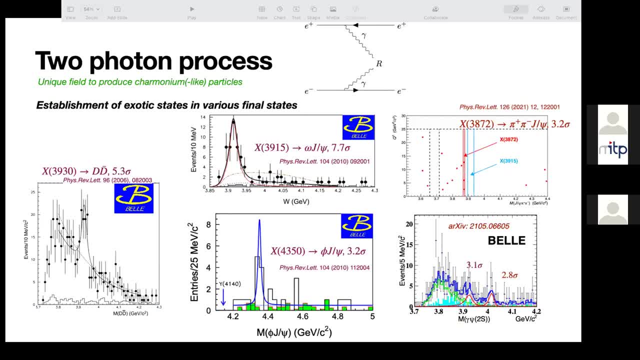 But the more consistent with the 3940, which is dominantly decayed to dd star. This is a remain puzzle to us. on the environment of Omega JSI. The X3950 was observed with the 7.7 Sigma. on the environment of 5 JSI. 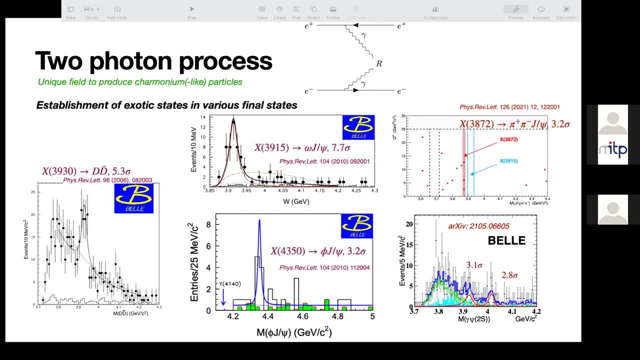 We. there is a no signal of Y4140, but evident of 4350 was observed was found Recently in the two photon process. the X372 signal decays to pi pi JSI was found as the evidence with the 3.2 Sigma. 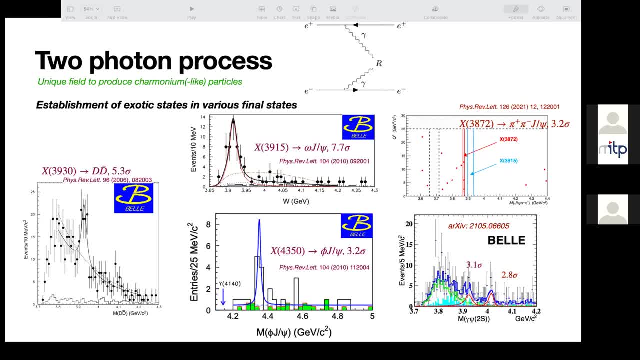 This, this: this tell us that the in the in the 2.2 process, the one or one or both of the two of the photons could be virtual in and the main provide a new mechanism to the to the X372 production. Recently, on the on the two photon process to 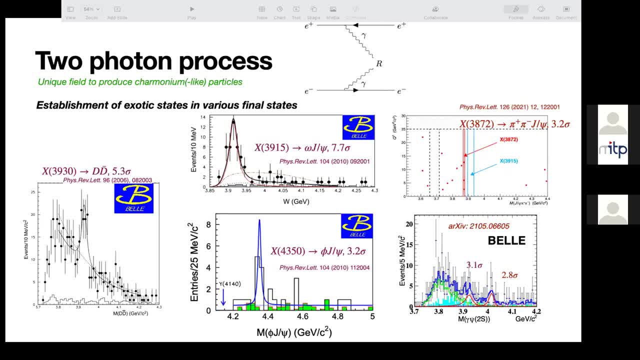 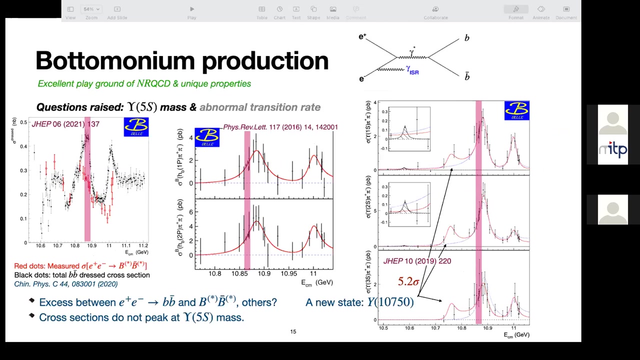 the gamma subprime. evidence of 3920 is found on the fund here and a new, a new, a new hint around for 4.02 GeV is found for the for the money production. This provide an excellent playground for the NLQCD. 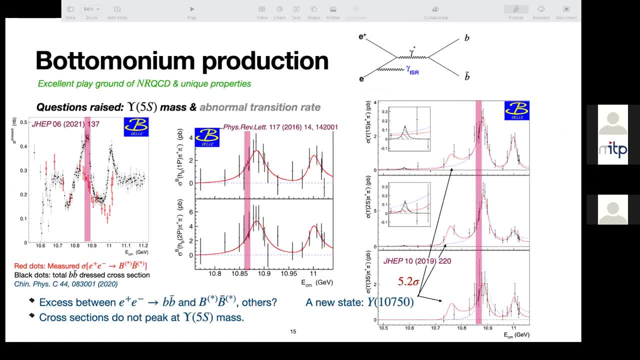 And for it also contains the unique properties. Firstly, a question will be raised: is the so-called Opsilon 5S? is what we believe, The what we the PDG number for the Opsilon 5S is The Opsilon 5S mass is the color of the pink bar on this, on this diagram. 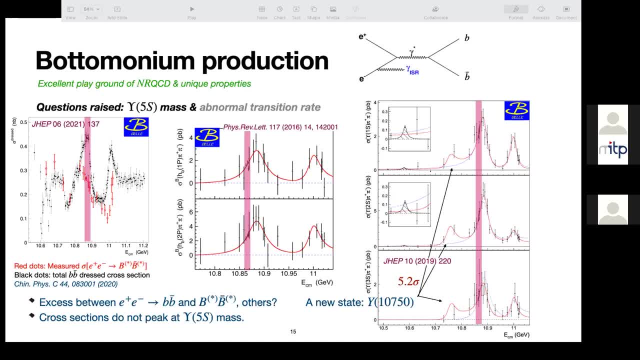 However, if you look at this left plot carefully, you can see that the peak value is not converged to the measured cross-section of the red dots, which is the measured cross-section of E plus, E minus goes to B star, B star, B star bar. 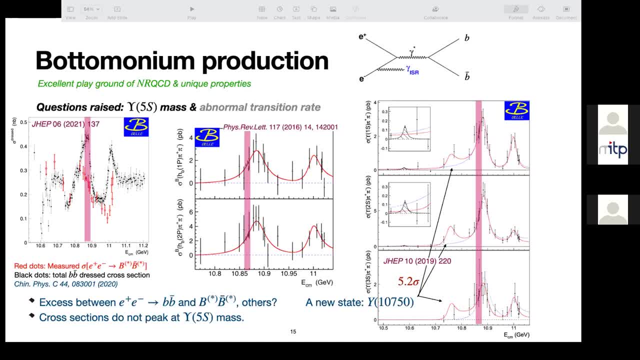 Well, the black dots are the total BB bar cross-sections. However, if you look at the other cross-section measurements, for example the middle plus the, which is the pi pi HB 1P and pi pi- HB 2P, the peak is on the. 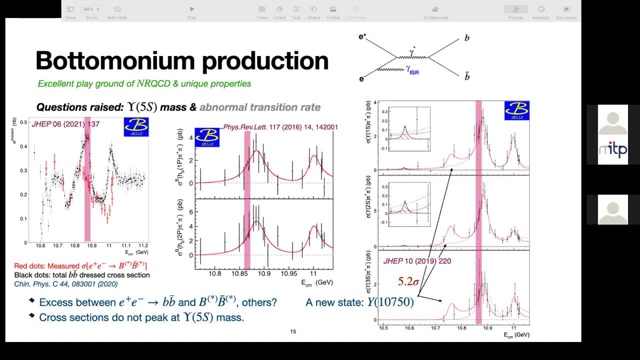 the peak of the cross-section is on the right of the so-called 5S mass. This is a similar peak is is found on the pi pi, Opsilon 1,, 2, 3S cross-sections. This this gives us a question that why these peaks are differently, but they are all close to the Opsilon 5S mass. 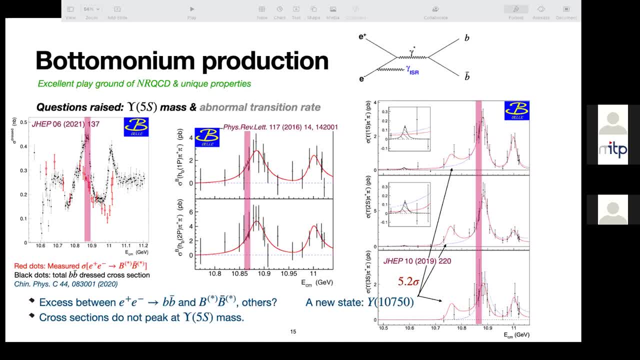 If we look at the left figure again- that you can- we can also see that there is an axis between the measured BB bar cross-sections and the B-methyl pair cross-sections. The axis comes from the BB bar, the B-methyl. 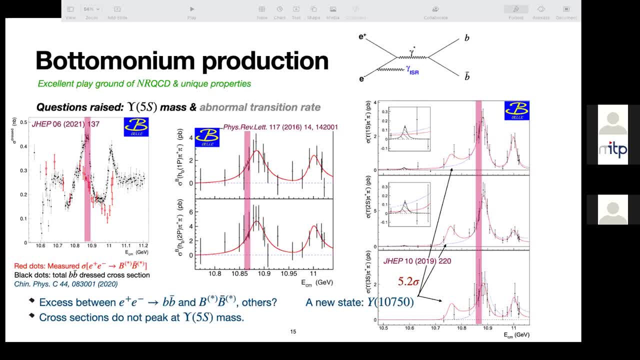 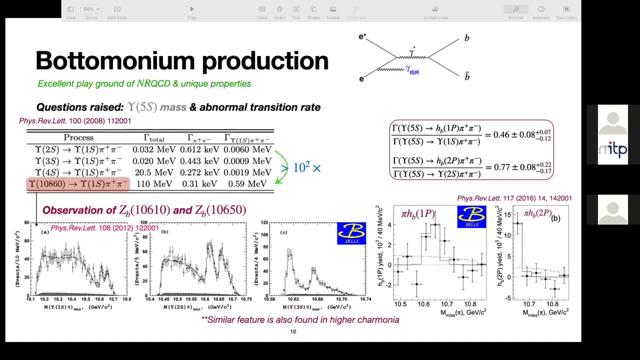 B-methyl pair with multiple pannels and the potassium transitions And this gives us a question that not question. This gives a very high abnormal transition rate for the bautimonium. From this figure we can see that the transition rate for the Opsilon 5S to pi pi Opsilon 1S is about 100 larger than the. 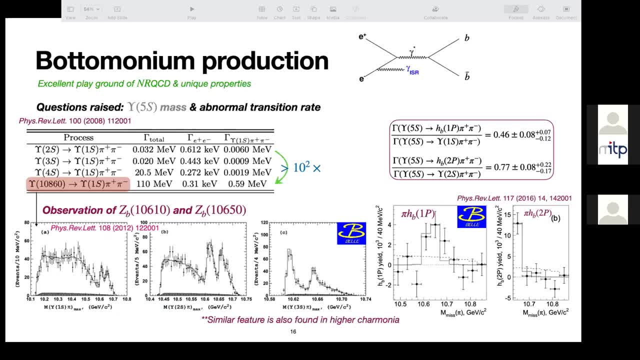 bautimonium below the open flavor threshold. This also leaves the observation of ZB 10, 6, 10 and 10, 6, 15.. This ZB state was also found in the pi pi HB transitions, which provide an essential contribution to this pi pi HB transition rate, because 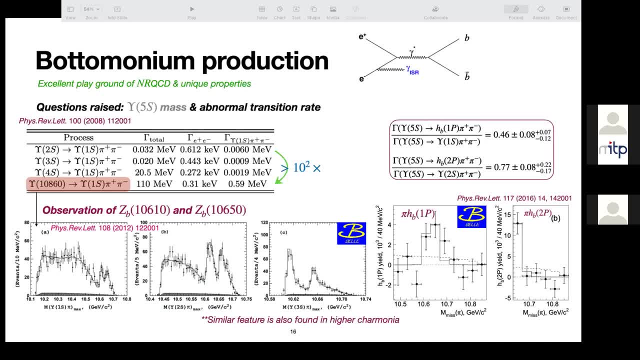 there is a spin flipped in this Opsilon 2 HB transition. Well, it should be. the transition rate should be very small. However, as you can see that this transition rate is compatible with the pi pi Opsilon, I would say that this similar figure is also found in the higher ammonium. 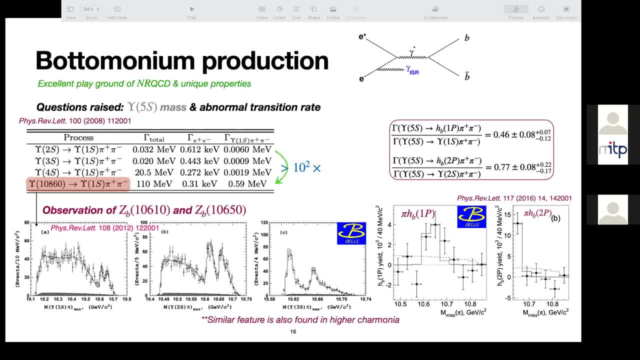 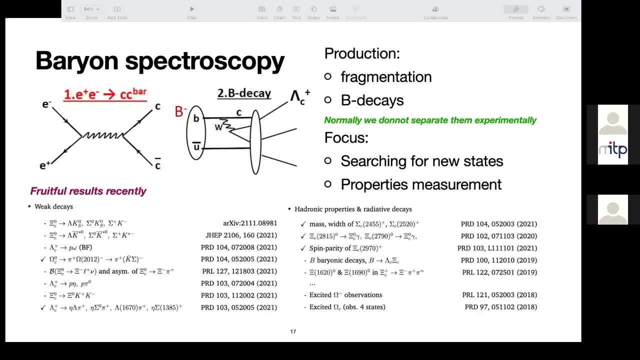 prior states, which also gives us a good view to better understand the correlation between the chamonium and the bautimonium states. Then let's move to the biance spectroscopy. The biance could be produced from the fragmentations and the BDKs. 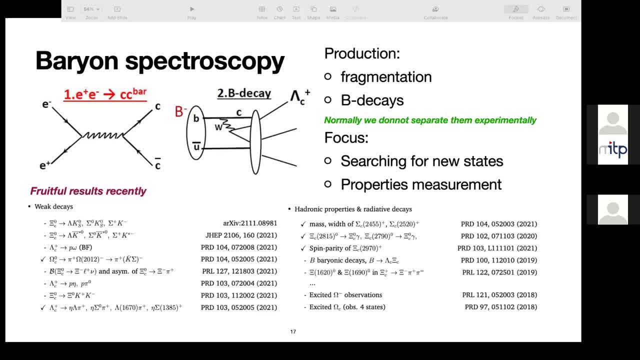 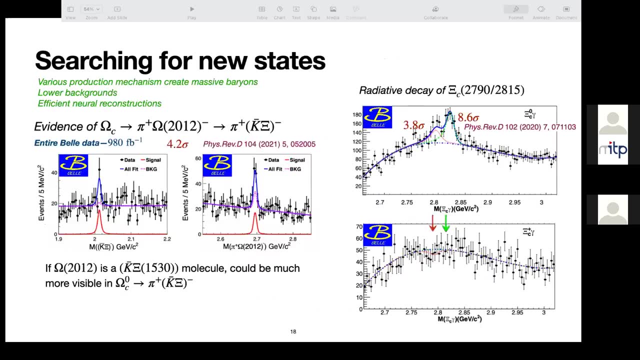 In this talk we will focus on the searching for the new states, on BAYO and the property measurements. Recently we have a fruitful results, but we will only focus on the few topics that we are list here. Firstly, the searching for the new state. 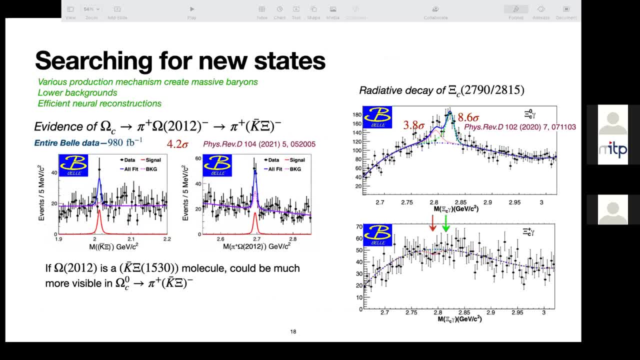 The various production mechanism will create a massive biance. The lower background by the E plus mass settings will also provide give us a good benefit to searching for The new states. Firstly, the evidence of the omega-c to pi, omega 2012.. 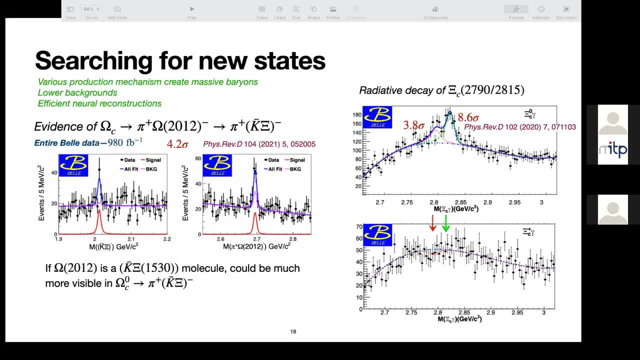 This omega 2012 was observed by BAYO And it is an, according to the theoretical calculation. If this is a KC molecular, it would be much more visible in the omega-c zero to pi KC And evidence is found in the two simultaneous. 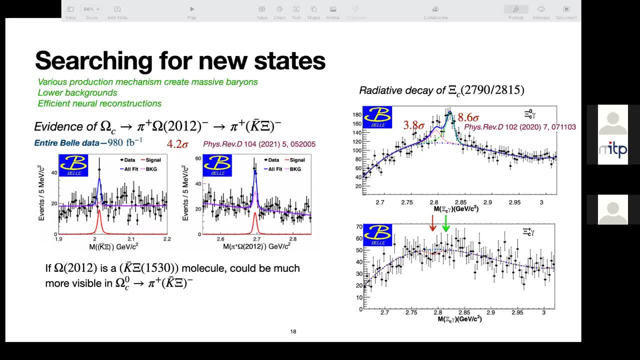 in the 2D simultaneous fit to the KC in random mass and the pi omega 2012 in random mass On the. the relative decay could also be searched on the BAYO because of the good reconstruction efficiency of the photons. Evidence of lower state are. 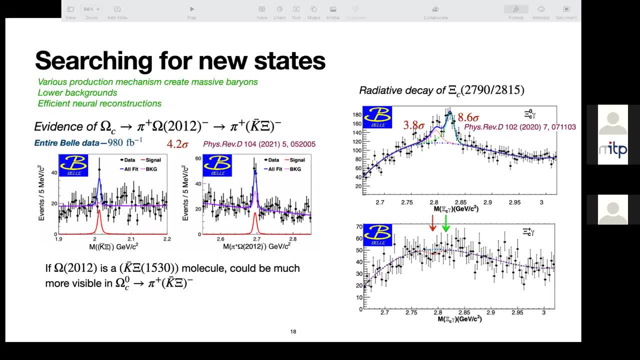 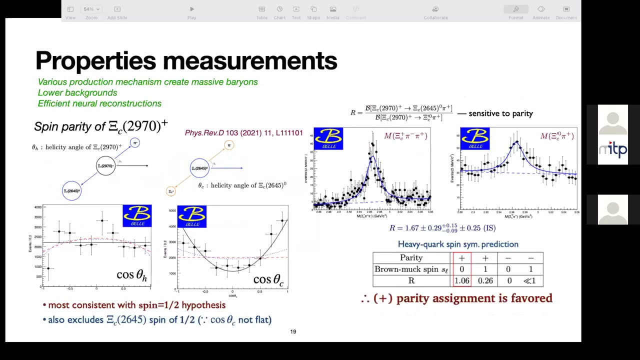 to to 20,, 27,000 was found on the environment of gamma KC, gamma KCC And and much high, much enhancement, much more enhanced. peak with, with observed near this small peak On the, on BAYO. 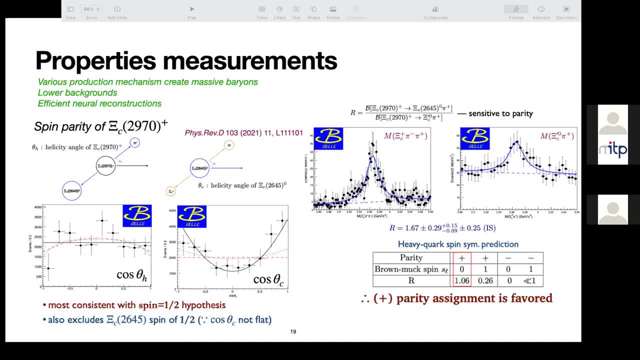 we can also do some property measurements, For example the spin parity. spin parity determinations: The spin could be determined by the helicity angle and the parity could be determined by the transition rate. On the left, two figures are the helicity angles of theta H and theta C. 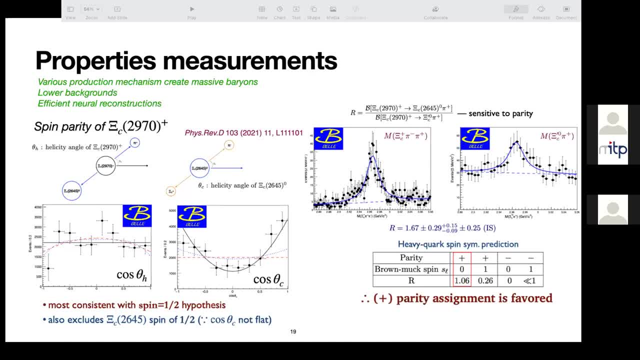 which is defined here, The most consistent. the fitted result is mostly consistent with the spin 1 over 2 hypothesis, And this is this also exclude KCC to 2600.. Now 20,, 26,, 45 spin over 1 over 2.. 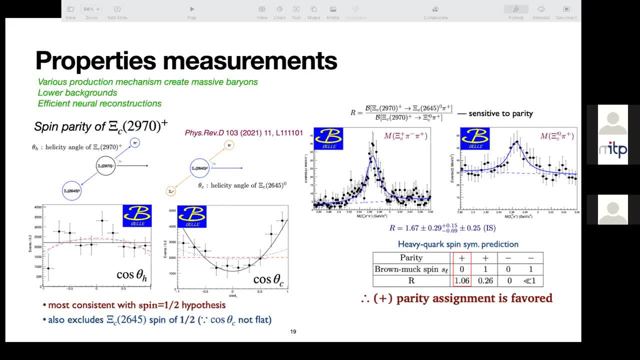 The ratio could be used to determine the parity, because it's this ratio is sensitive. According to the theoretical calculation, the, this ratio would be very close to 1.06 and, compared with the experiment calculation, this positive parity is assigned to this particle. 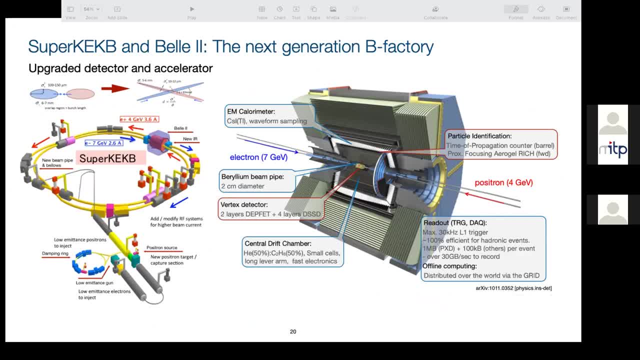 Then let's move to the SuperKey KB and BAYO2.. SuperKey KB and BAYO2 is a next generation prefactory. We have upgraded detectors and accelerator. With the benefit of a nano beam, we can have almost 30 times integral. 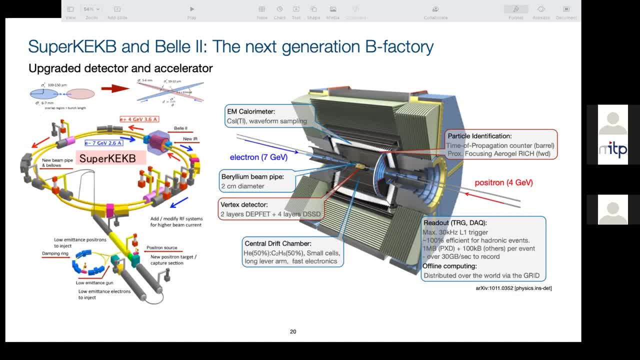 larger integrated, not sorry, 30 times larger instantaneous luminosity and almost 40 times of integrated luminosity For the BAYO2, we the track per system is upgraded and so as so as the KOM and the software part. 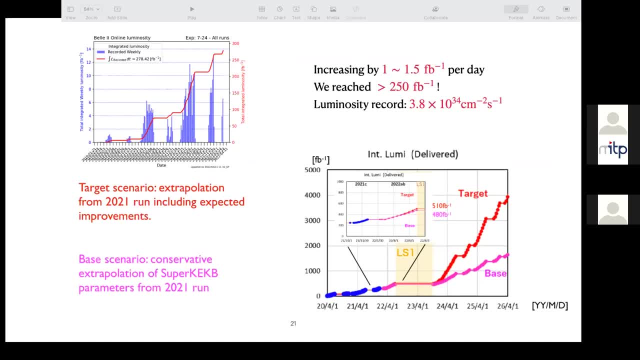 By now, the we have already achieved 250 inverse KB and the luminosity is increasing by 1 or 1. 1 to 1.5 inverse KB per day. The maximum luminosity record is the 3.8 times 10 to 34.. 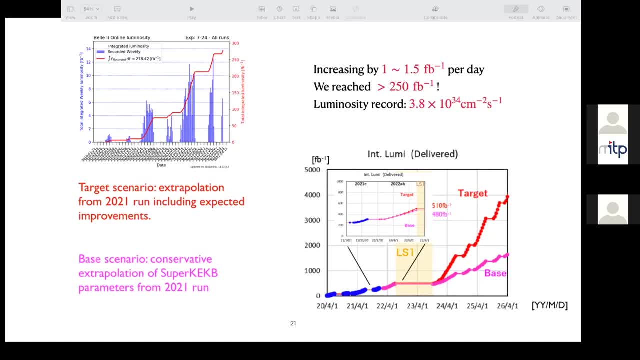 The target of the summer of this year. we will have a large shutdown To upgrade the detector. we target to have a 500 inverse figure bar data at that time And the baseline is 480 inverse figure bar. Here is our prospect. 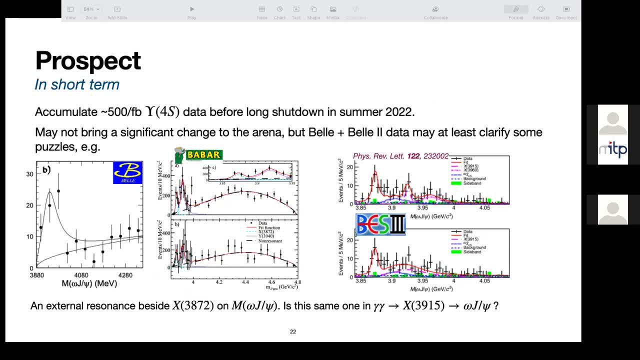 In short term actually accumulate around 5 inverse figure bar of epsilon s before. the long shutdown in before the summer of this year may not bring a significant change in to the arena, But if we combine BAYO and BAYO2 data, 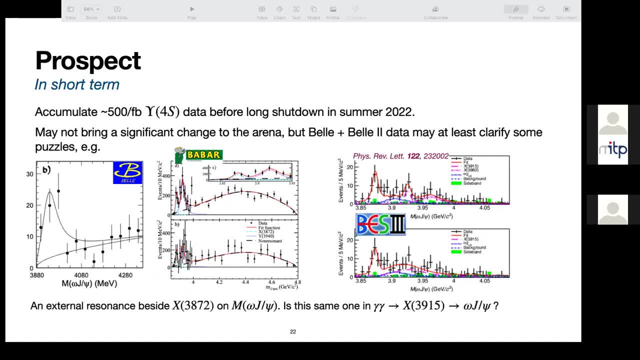 we may at least clarify some puzzles. For example, there is an extra resonance beside X3872 on the environment mass of omic JSI. This is the firstly clarified. This is the first claim, firstly claimed by BAYO and BAYO2.. 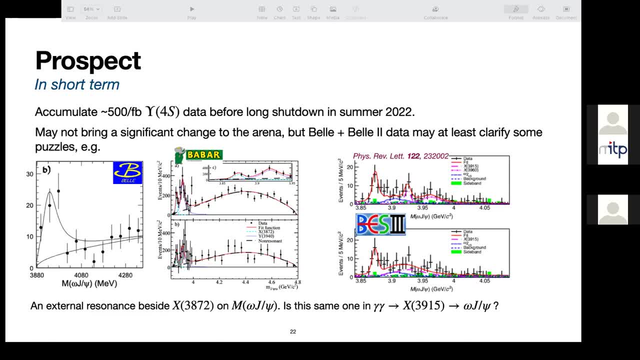 And recently the BAYO3 published the environment mass, the study of omic JSI. But it's very difficult to tell whether this is the one, whether they are one particles or two. So if we have an extra 500 data, 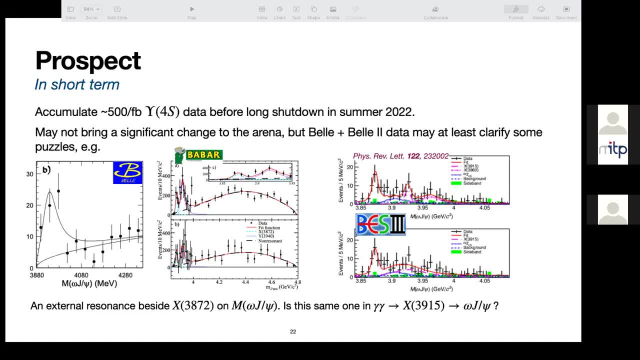 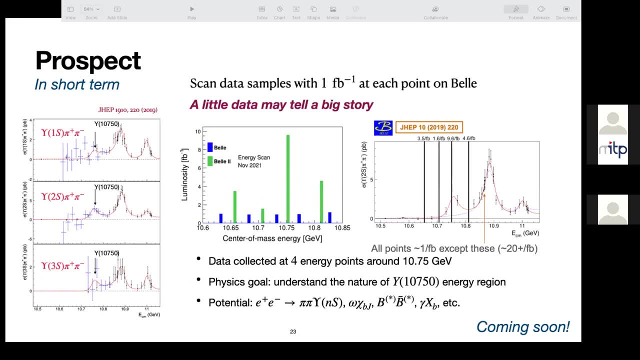 we could at least say something on this. Another prospect is a new. a new white state is observed in the pi pi epsilon environment mass around 10.7, 75 GV. However, limited by the luminosity, there is only like one inverse figure bar at each scan point on BAYO. 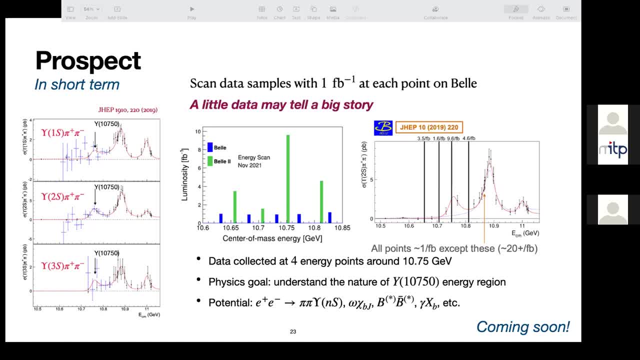 Based on that, if we have- even we have- a little data, we can tell a big story on this new state, Unless on November last year. in November last year we have an energy scan around 10 point at the peak of 10.75 GV, and also three points. 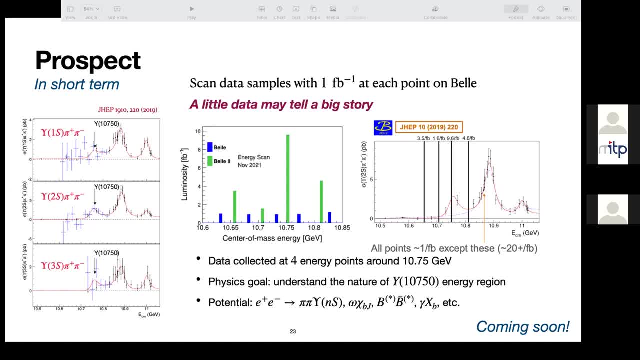 three points around this, this, this energy. In total we have like 20 inverse figure bar datas. The physics goal would be understand the nature of this: Y, 10,, 7,, 50.. And there are several potential analysis, For example: 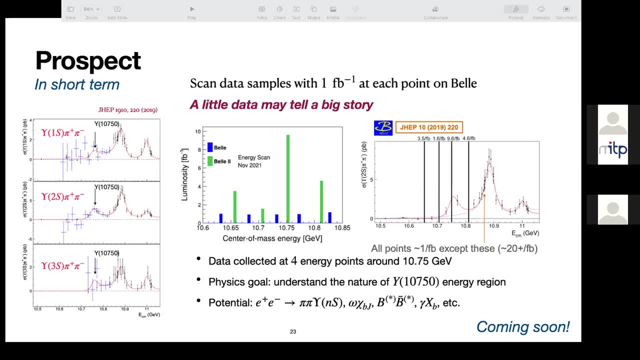 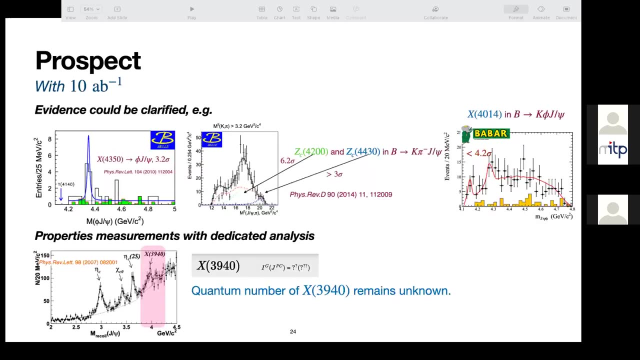 E plus, E minus go to pi pi epsilon and omega KB B meson pair, B star meson pairs or gamma XB studies And the result will come in soon. If we have, we, if we can accumulate 10 inverse figure bar data. 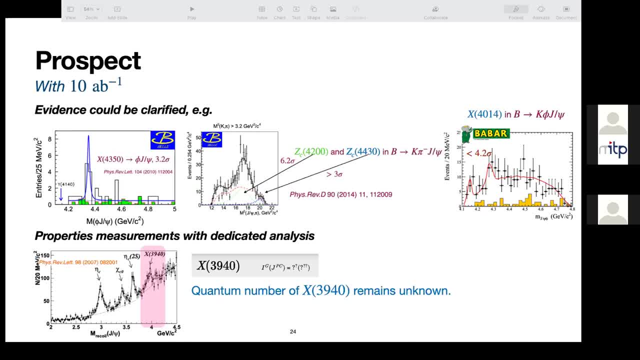 we can. we can clarify some evidence, that raised by Bill and other experiments, For example on the environment of 5G side. we can have a better understanding of this particle to confirm or reject this hand. This is this particle And also some other. 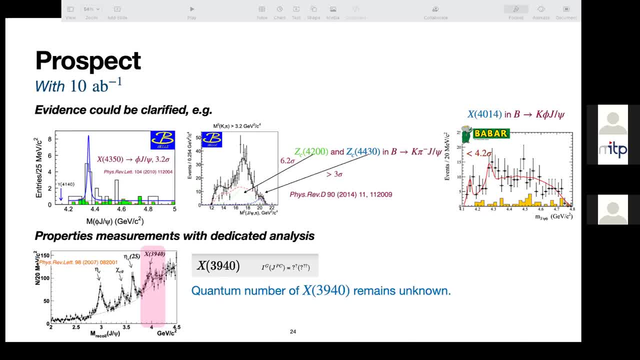 these particles in the, in the waves, also help to determine the spin parity. So from to the biomass of this you can go, you know. okay, so we can also use the spin parity evidence to estimate this, this, this, this energy index, to also determine the spin parity of those. 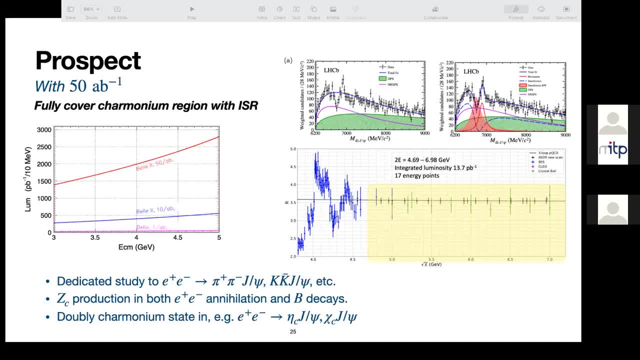 the, the, the energy index of this particular particle. So, for example, let's say here, let's say here, let's say a, we can fully cover the Chamonix region with ICR process, A dedicated analysis to the E plus, E minus to Piper JSI. 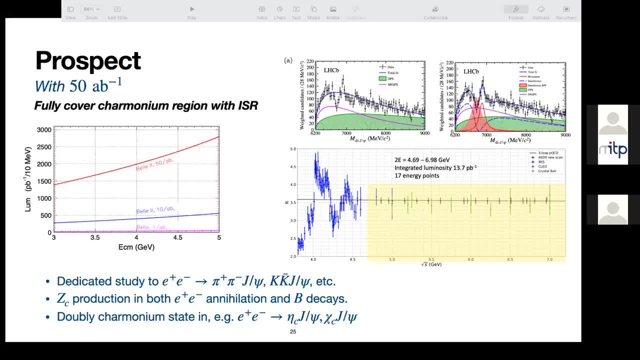 KK, JSI or other Cham-Beyond pairs production regions. The ZC production in both E plus, E minus annihilation and BDKs will also give us a good understanding to these natures. The W-Chamonium states production could be also covered. 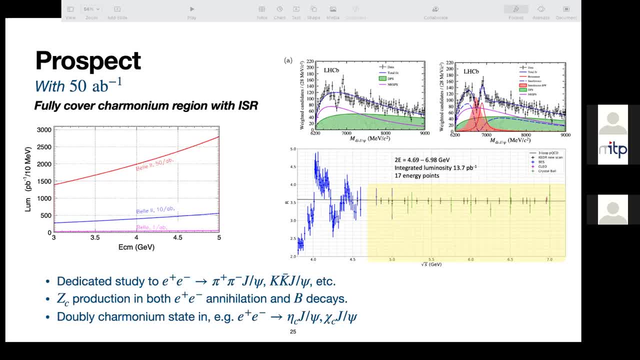 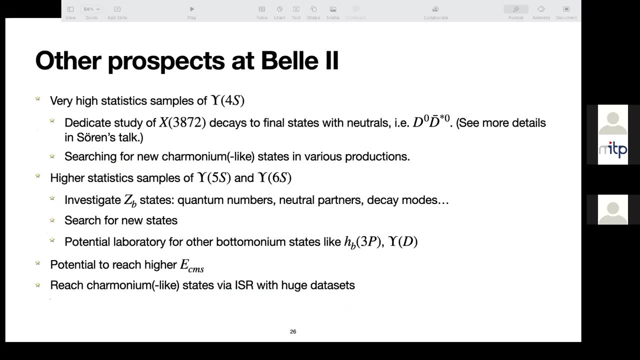 in the ICR region for example. for instance, the E plus, E minus go to ETC JSI or KC JSI. For other prospects at BIL2, we could have very high statistical statistics. samples of OOPSON4S. 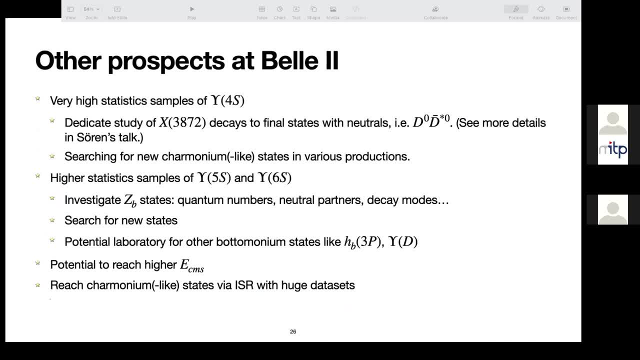 A dedicated study of X372 decayed to the final state with neutrals would be very interesting, For example the D0, D0 star. You can check more details in Soren's talk after a few days. We can also search for some new Chamonium-like states. 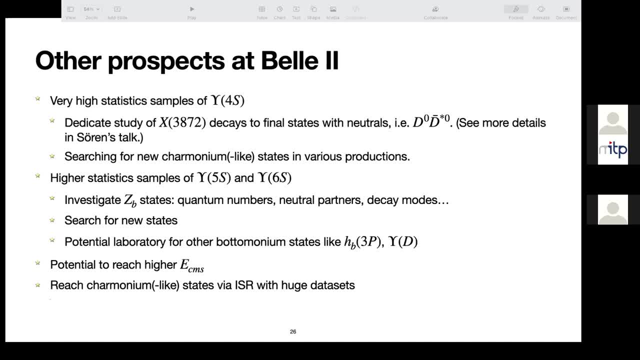 in various productions or the amplitude analysis. The higher statical samples over the OOPSON5S and OOPSON6S will allow us to investigate the ZB states, including the quantum numbers, neutral panels, decent moves. We can also search for the new. 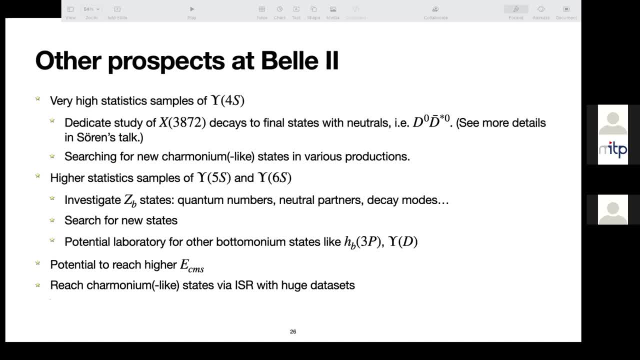 좋almonium-like states and we can also these large OOPSON5S or the OOPSON6T noiseiße data whoops on five and success states can also provide a potential laboratory for other portfolio states like hb or oops on these days, and the bill tool is also potential to reach higher. 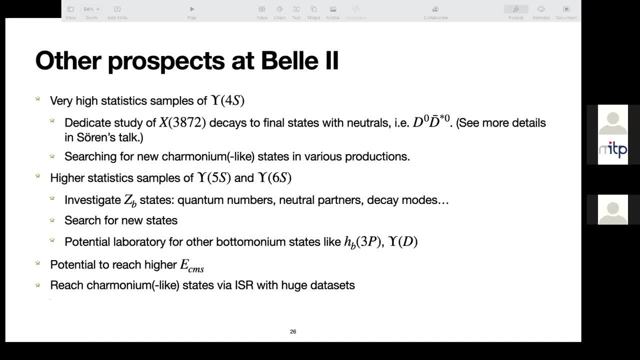 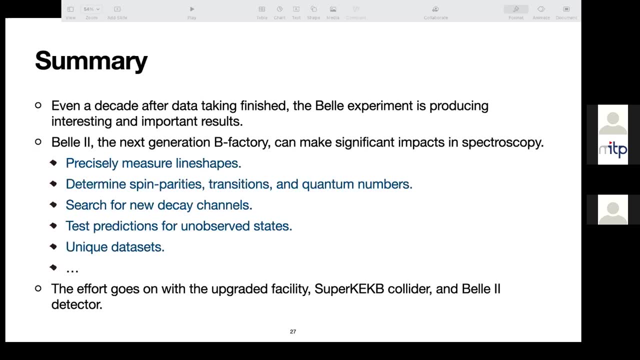 center of mass energy, for example, the lambda b, lambda b pi, lambda b lambda, lambda b, bar pair region. uh, in a summary, uh, even a decade after data ticking finish, the bill experiment is still producing interesting and important result. built to the next generation b factory can make 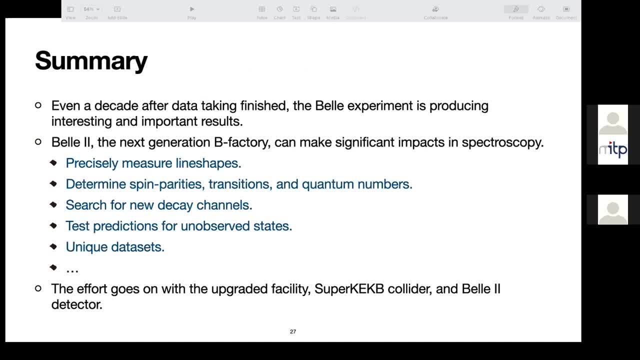 significant impact in the spectroscopy, including, but not limited to the precise lunch shape measurements, quantum number determination, that for new decay channels or new states and so on. the efforts will goes on with the up to upgraded. still goes on with the upgraded facilities over kkb's collider and built to detector. okay, that's all, thank you. 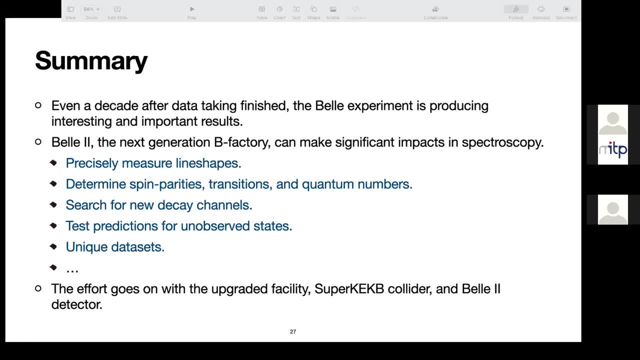 thank you for this very nice overview. we are open for questions and comments. thank you for this very nice overview. we are open for questions and comments. thank you for this very nice overview. we are open for questions and comments. yes, please, yes, it's a me, okay. yeah, let me see, i wanted to make a comment, i mean again. 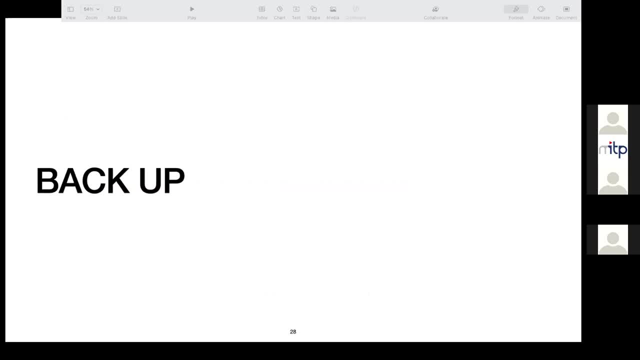 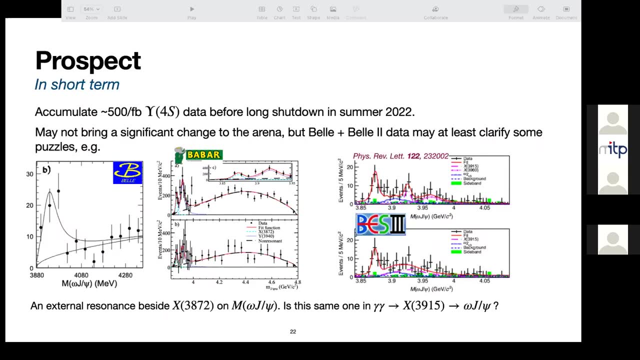 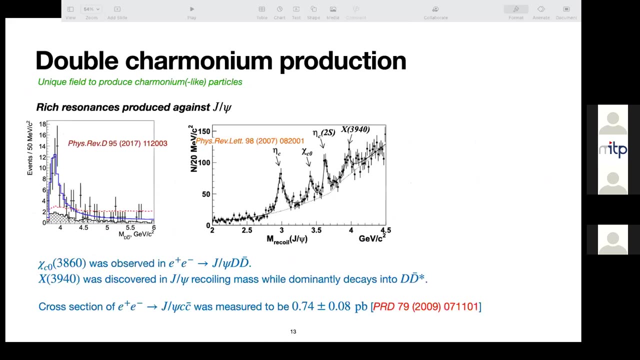 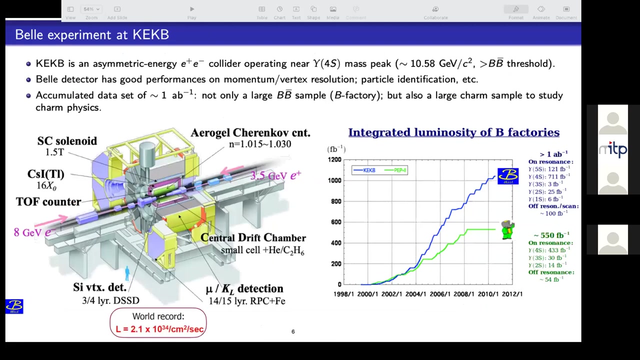 in page 13 you have the talk again a bit about this tc0 3860 that i made a comment before when the lhcb talk was given. i think i mean lhcb. yeah, lhcb has ruled out that state. yeah, uh, page 13, page 13, 13, 13, 13. sorry, i have something wrong with my computer. please. 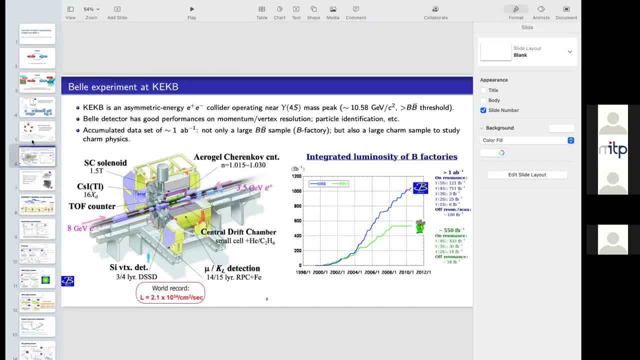 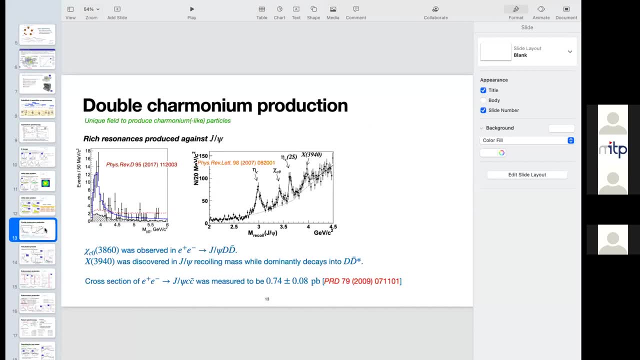 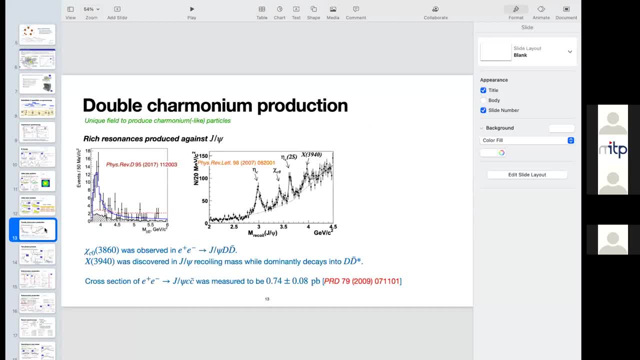 no, no, i think. i mean. i think i mean after the observation, i mean in the very good analysis with the data of hcb. you should not claim that anymore. i think you should remove the claims for that. apart from the work that we what? apart from the work that i have always? i have mentioned before. 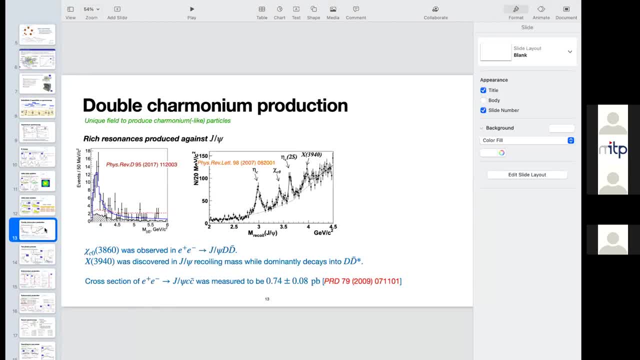 there is an excellent work right now from mark van der heaven analyzing gama gama by going to dd bar. well, it was also claimed that state and they see again that there is no, no signal at all of that state. So I think please, I mean I would advise you. 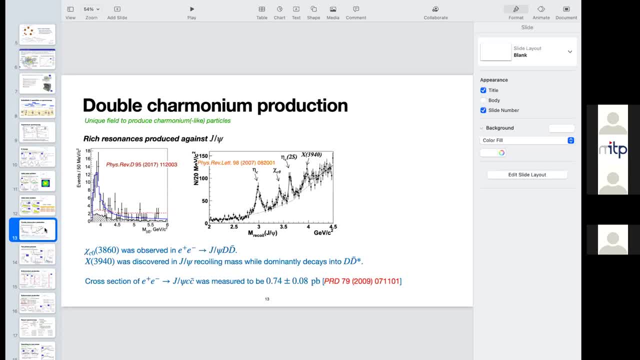 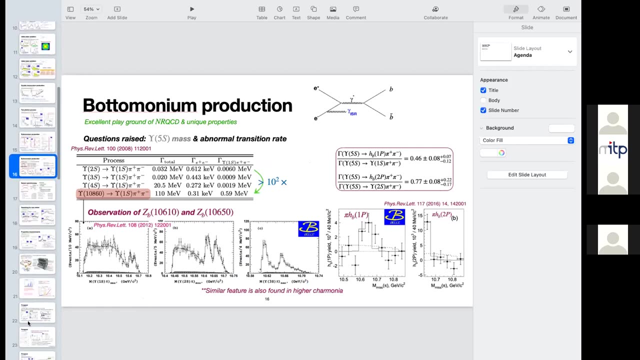 just to remove the claims. There is no reason for that anymore. Okay, now I mean in the page 18, page 18, you have something there concerning the Omega 2012, which I think you have made a mistake in the writing. 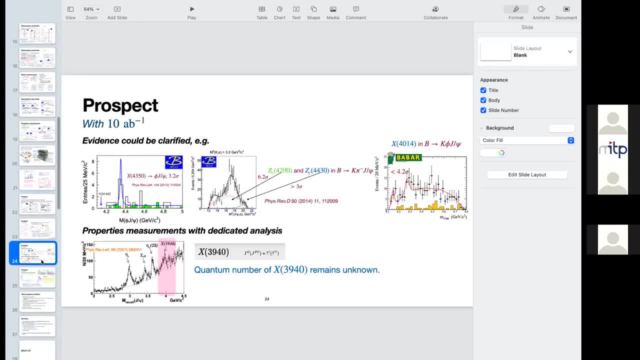 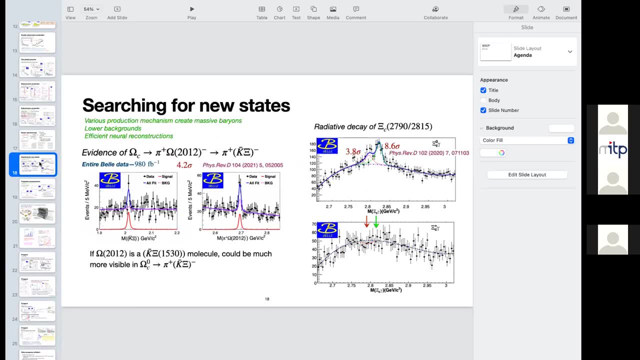 I mean, I tell you, I mean, but I think there is a mistake in the writing, because 18, page 18, one eight. yeah, You see that if it's a molecule could be much more visible in Omega C, pi plus no. 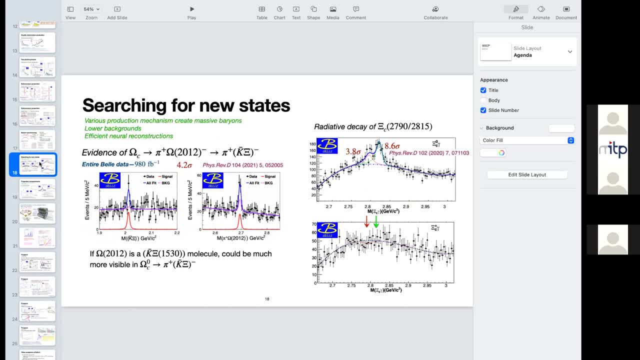 because one pi plus comes from the V decay and then you have the Omega 2012 decay, which can decay into K bar cascade or K bar cascade bar, and then there is a K bar cascade pi. So there are two pions. so this is not well written. 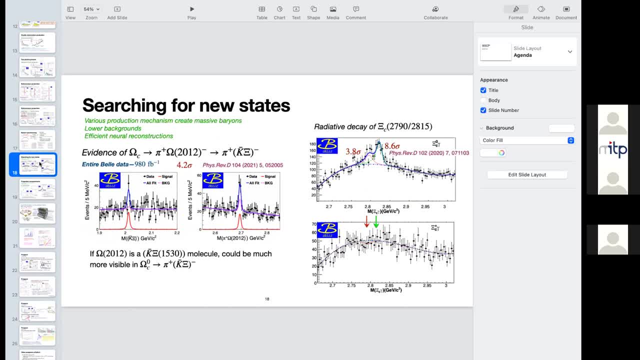 And in any case, you know, I want to mention, I mean there are two independent works. One is by Xie Zhijun, and you see colleagues of yours, Xie Zhijun and Lixian Geng. 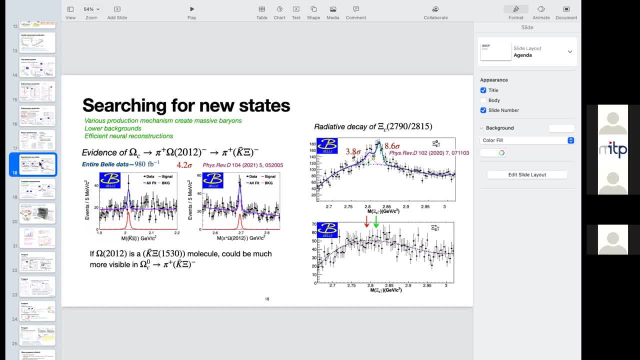 and independent is one from Toledo and Hino in which they show, I mean, that there is no problem. The data of Bell, I mean, can be explained within the framework of the molecule, Two independent works. they agree on the conclusions. 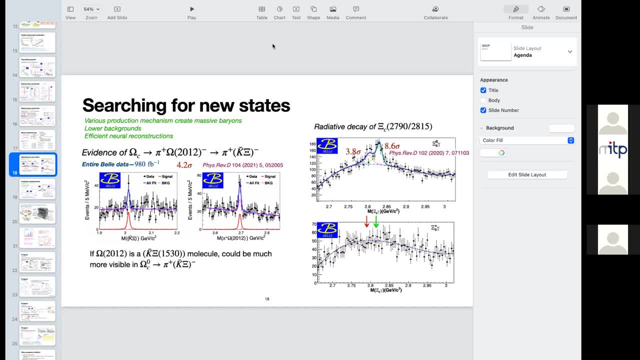 And finally, to finish, I mean one recommendation. you know I would recommend I mean the Bell collaboration, particularly all experimental, But particularly the Bell collaboration to provide the data which are efficiency corrected. You said in the introduction how important it is. 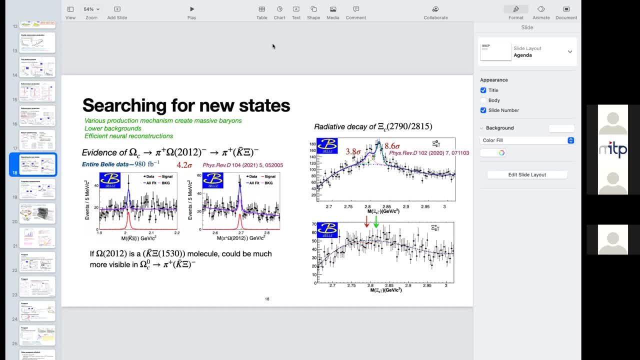 that it is. I mean work, I mean between theory and experiment. If you don't give us the data which is efficiency corrected, we cannot compare. So, and you know, my experience is that all the data that I had I mean to have been reproduced from Bell. 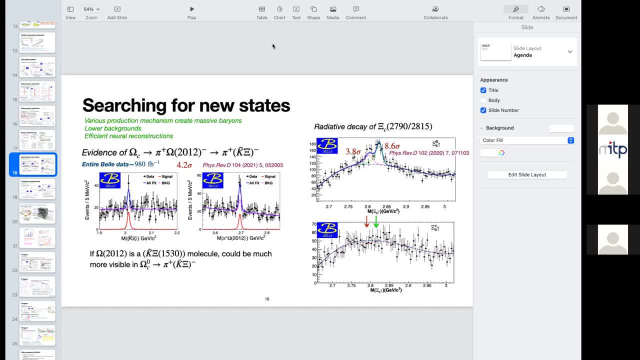 all of them. I mean, were not efficiency corrected? Some people have been nice- I mean too in private, give me the corrected data And others laugh at me. even you know I mean they had I mean the shame of laughing at me. 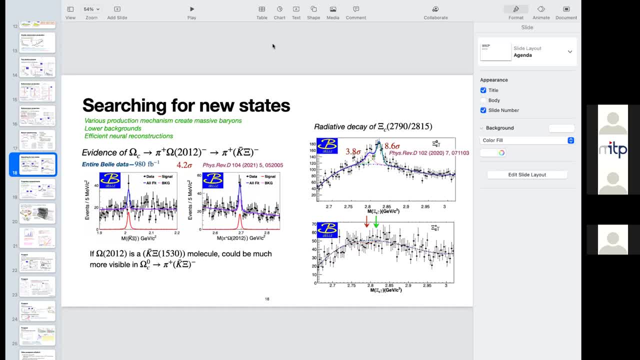 saying that I could not reproduce the data because they were not efficiently corrected. That is something insulting, because you know I mean. the first thing I mean of an experiment is that it should be reproducible, And if you don't give us the data, I mean 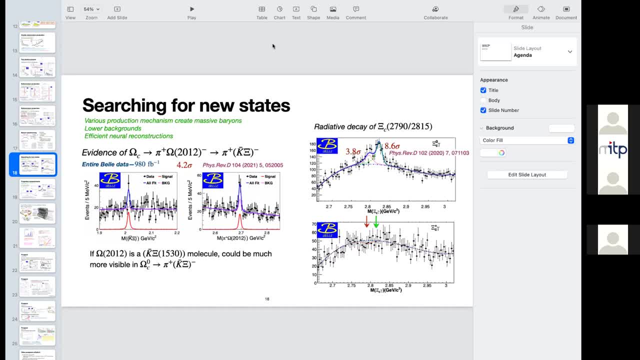 which are efficiently corrected. I mean, we cannot reproduce it, Okay. so I mean please take that into consideration and make a favor to us theoreticians and to the community to give the data. Yeah, I think this is a general comment. 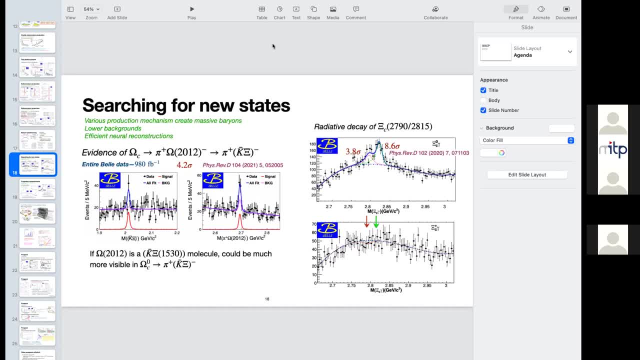 to all the good environmentalists, not for this part only. This is correct. but I mean, at least you know I have had the same experience with the LHCV, But the LHCV at least they were giving me. I mean. 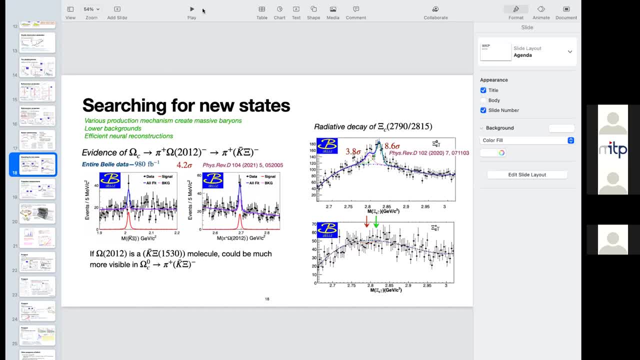 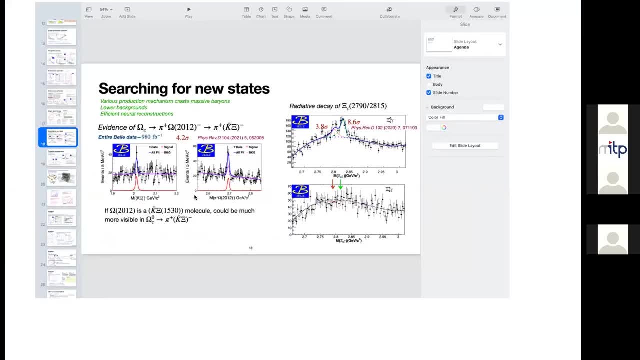 the data with the phase space. Phase space I mean correct, I mean with the efficiency, I mean I mean that they had And then from there I could reproduce. I mean the data efficiently corrected. But I mean that I did have a bit of a chance. 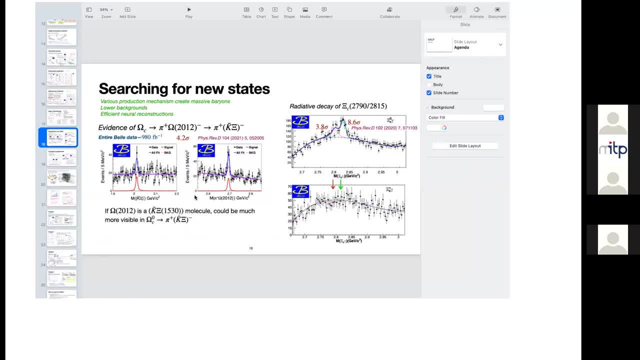 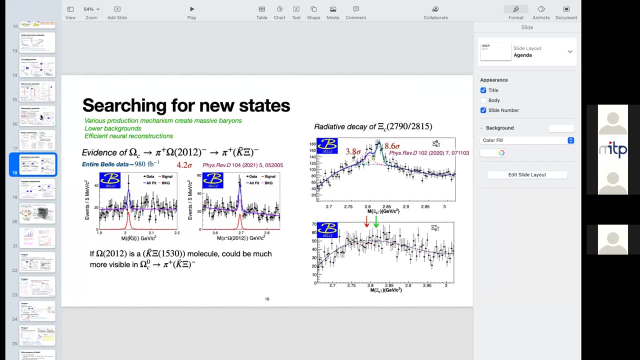 I mean with a bit of data, I know. Okay, thank you for the comments, I think. is there any other questions? comments to this talk? I have one question. You mentioned the typical category kind of, in principle, run at a higher energy. 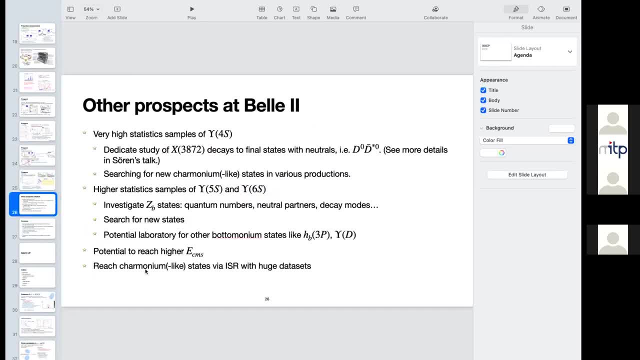 So how high can it take a DOH? Yes, so currently we don't have some numbers on this estimation, but this is just an approved proposal. Yes, just a proposal to the accelerator side that we want to have a higher energy to the, for example. 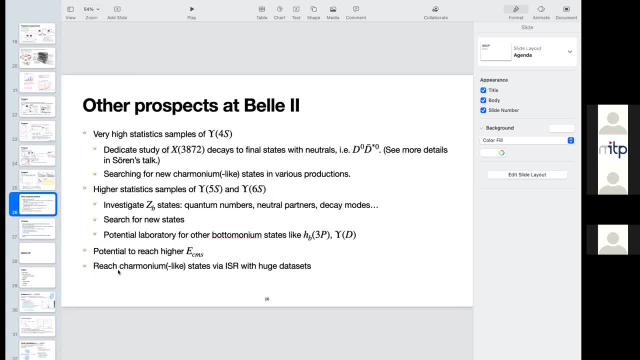 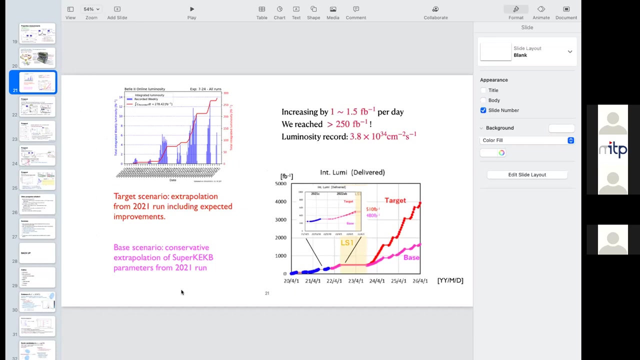 lambda B. lambda B bar NG region. Okay, I'm reading your slide, the 21.. You mentioned the short term plan to accumulate 500 and use data. Yeah, this is Yeah. yeah, this is the plan. I just wonder: how is this 500 in the federal bar data?